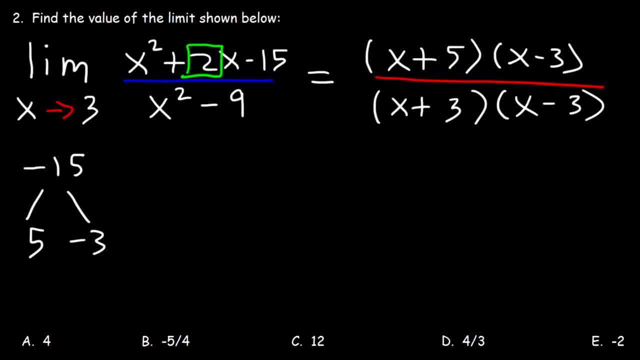 One of them is going to be plus, the other is going to be minus. Notice that we can cancel x minus 3.. So now we can evaluate the limit as x approaches 3 of x plus 5 divided by x plus 3.. 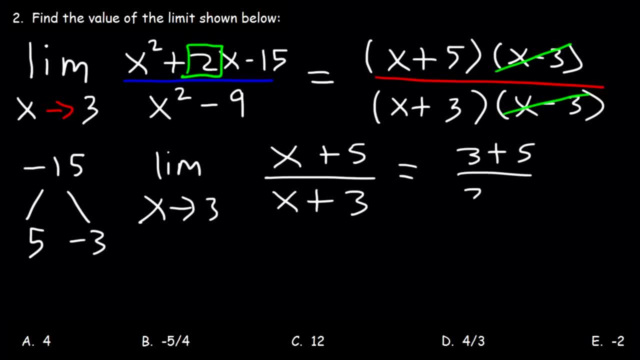 So it's going to be 3 plus 5 divided by 3 plus 3.. And so that's 8 divided by 6, which reduces to 4 divided by 3 if you divide both numbers by 2.. So therefore, d is the right answer. 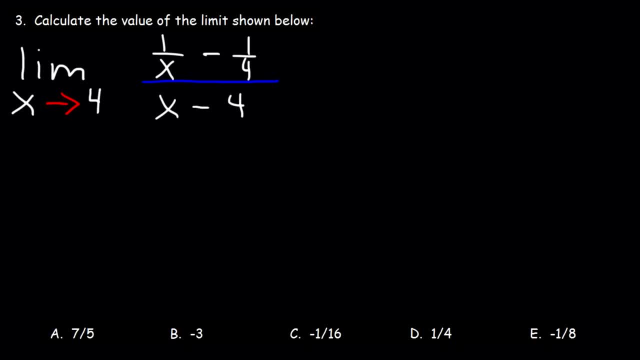 Number 3. Calculate the value of the limit shown below. So, whenever you have a complex fraction, what you want to do is multiply the top and the bottom by the common denominator, The common denominator being 4x. So on the top, you want to distribute. 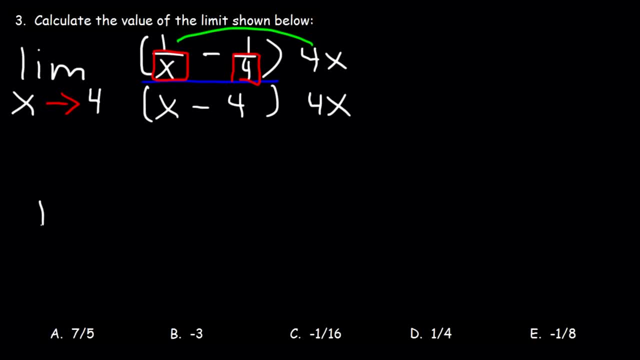 4x times 1 over x is 4.. 4x is the same as 4x over 1.. And you can see, the x variables will cancel, leaving behind 4.. So, therefore, what we now have is the limit as x approaches 4.. 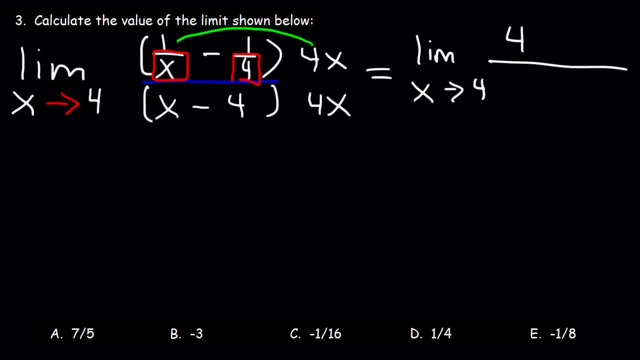 And on top we have positive 4.. Now if we multiply 4x by 1 over 4, you can see that the 4s will cancel, leaving behind x, And there's a negative sign in front. So it's going to be minus. 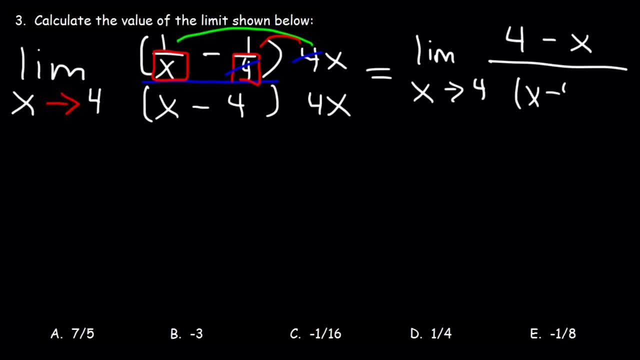 Minus x, And on the bottom we're just going to rewrite x minus 4 and 4 minus x. Now these two factors look very similar, but they're not exactly the same. So what we're going to do is we're going to factor out a negative 1.. 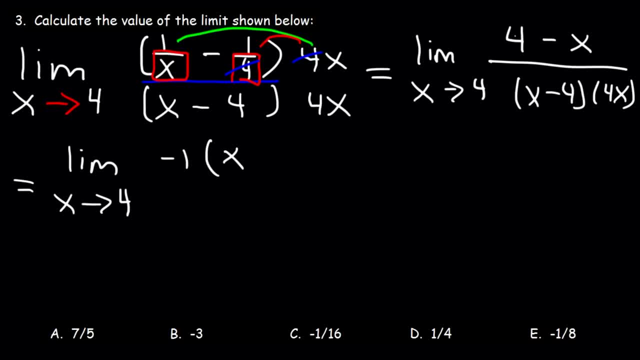 If we do so, negative x will change into positive x, And positive 4 will change into negative 4.. And it's at this point that we can get rid of the x minus 4.. So now we have the limit, as x approaches 4, of negative 1 divided by 4x. 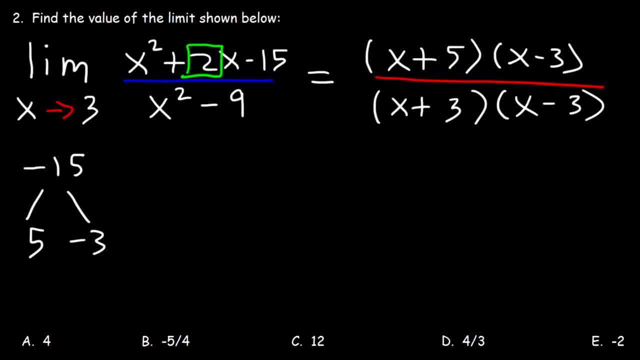 One of them is going to be plus, the other is going to be minus. Notice that we can cancel x minus 3.. So now we can evaluate the limit as x approaches 3 of x plus 5 divided by x plus 3.. 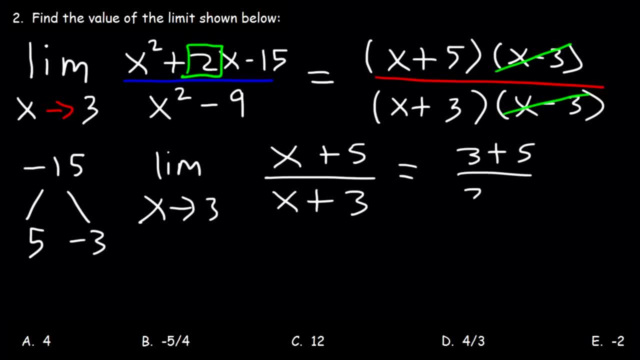 So it's going to be 3 plus 5 divided by 3 plus 3.. And so that's 8 divided by 6, which reduces to 4 divided by 3 if you divide both numbers by 2.. So therefore, d is the right answer. 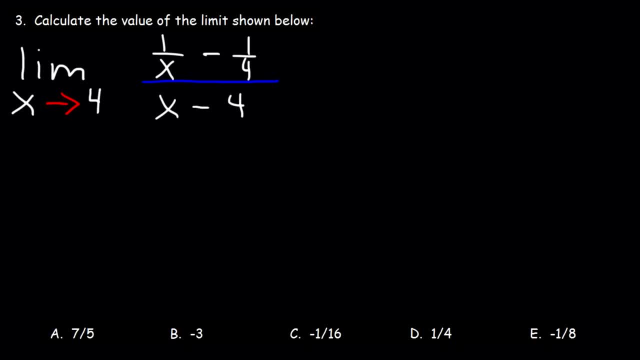 Number 3. Calculate the value of the limit shown below. So, whenever you have a complex fraction, what you want to do is multiply the top and the bottom by the common denominator, The common denominator being 4x. So on the top, you want to distribute. 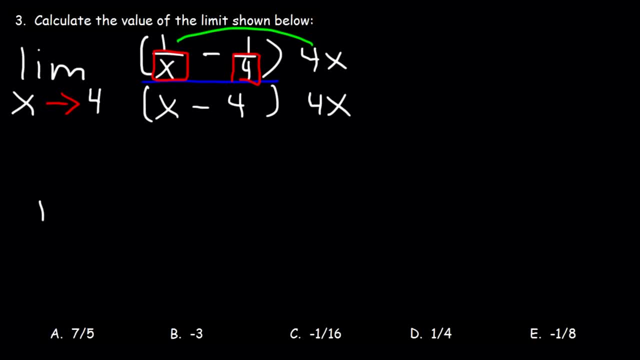 4x times 1 over x is 4.. 4x is the value of the limit shown below. 4x is the value of the limit shown below. 4x is the same as 4x over 1.. And you can see the x variables will cancel, leaving behind 4.. 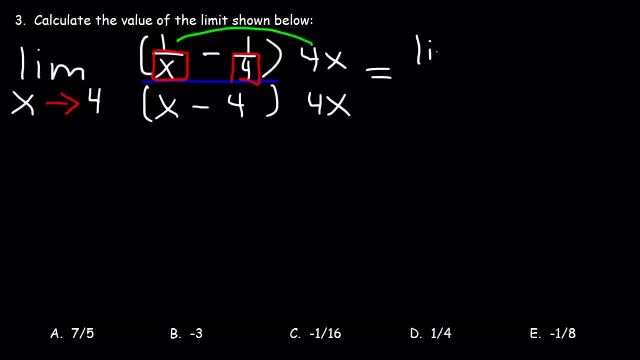 So, therefore, what we now have is the limit as x approaches 4. And on top we have positive 4.. Now, if we multiply 4x by 1 over 4, you can see that the 4s will cancel, leaving behind x. 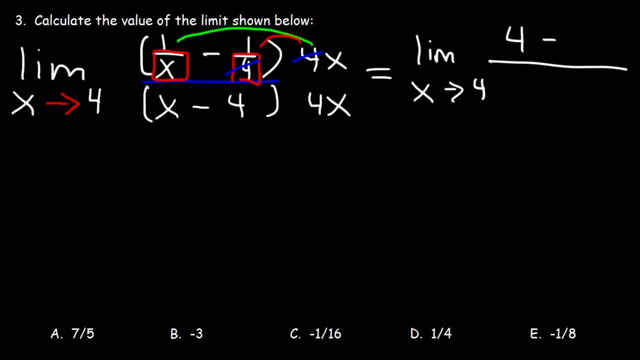 And there's a negative sign in front. So it's going to be minus x And on the bottom, we're just going to, We're just going to rewrite x minus 4 and 4 minus x. Now these two factors look very similar, but they're not exactly the same. 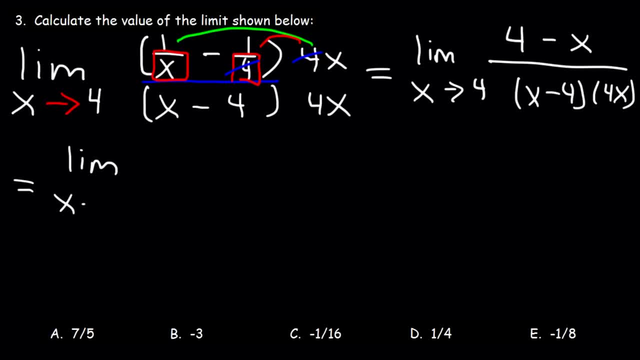 So what we're going to do is we're going to factor out a negative 1.. If we do so, negative x will change into positive x, And positive 4 will change into negative 4.. And it's at this point that we can get rid of the x minus 4.. 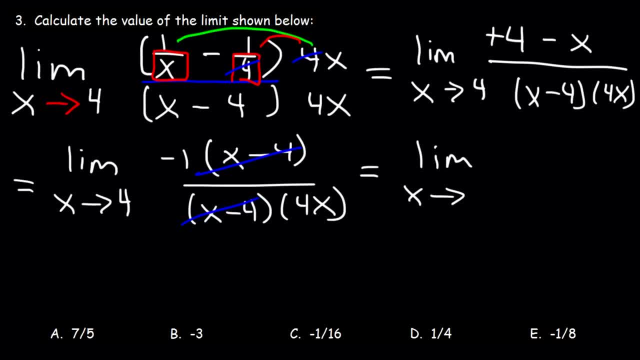 So now we have the limit, As x approaches 4, of negative 1 divided by 4x. now we can use direct substitution. So this is going to be negative 1 over 4 times 4, which gives us a final answer of negative 1 divided by 16.. 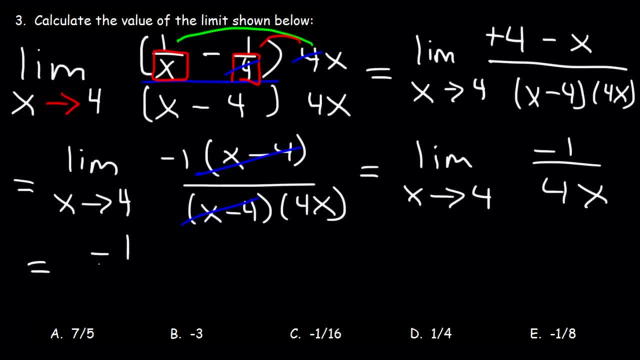 Now we can use direct substitution. So this is going to be negative 1 over 4 times 4, which gives us a final answer of negative 1 divided by 16.. Which means c is the right answer, Number 4.. Find the value of the limit. 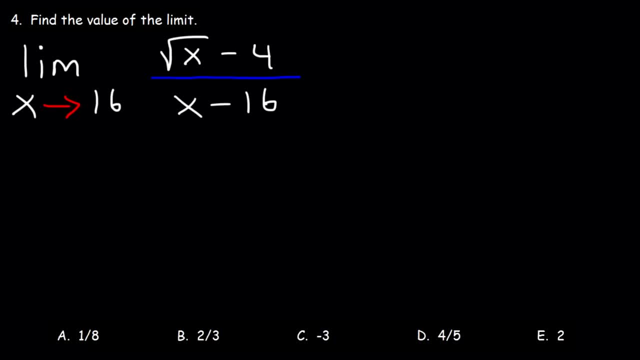 So here we have a rational function with a square root on the top. In a situation like this, you need to multiply the top and the bottom by the conjugate of the numerator. The conjugate is going to be the same thing, but you've got to change the negative sign into a positive sign. 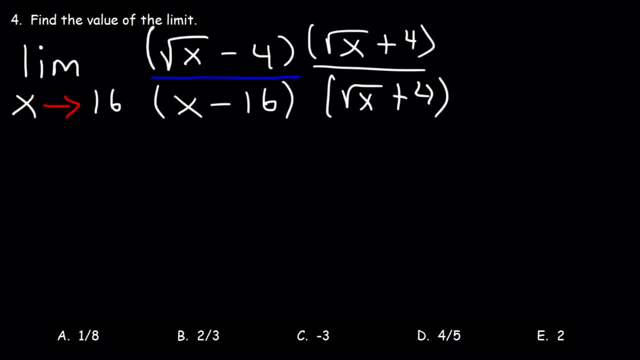 And whatever you do to the top, you must also do to the bottom. Now, on top, we're going to FOIL The square root of x times the square root of x is equal to x, The square root of x times 4.. 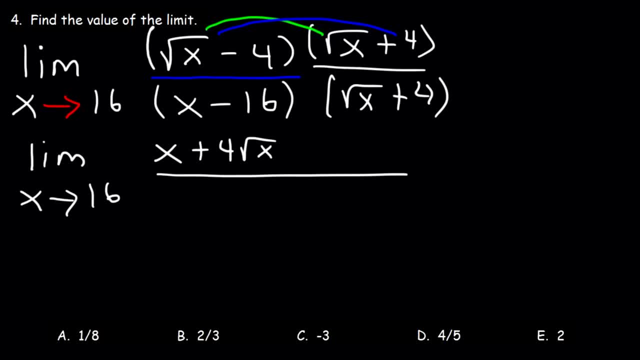 That's going to be x. That's going to be positive 4 square root x And negative 4 times the square root of x is going to be what you see here. And finally, we have negative 4 times 4, which is negative 16.. 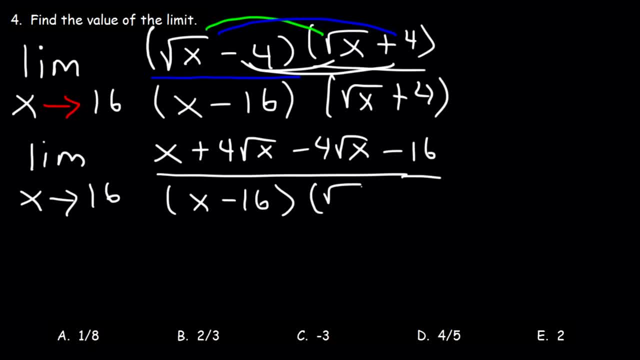 In a denominator. we're not going to FOIL, We're just going to rewrite what we have, So we can see that the two middle terms add up to 0. And they're going to disappear. So now what we have is the limit, as x approaches 16, of x minus 16 divided by 16.. 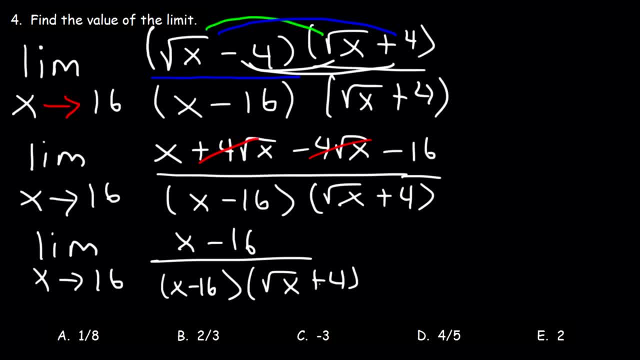 x minus 16 times the square root of x plus 4.. So now we can cancel x minus 16.. And at this point we can replace x with 16.. So this is going to be 1 divided by the square root of 16 plus 4.. 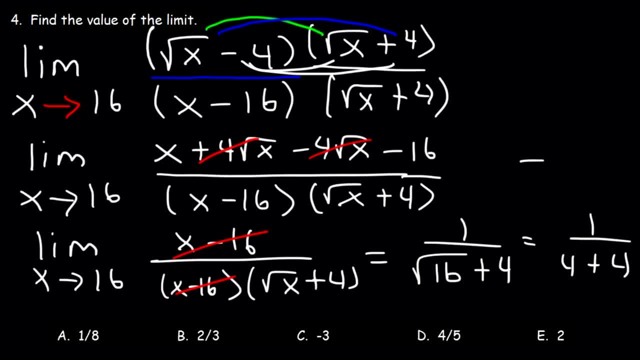 The square root of 16 is 4. And 4 plus 4 is 8.. So the answer is 1 divided by 8, which corresponds to answer choice A Number 5.. Evaluate the limit, So we can't plug in 7.. 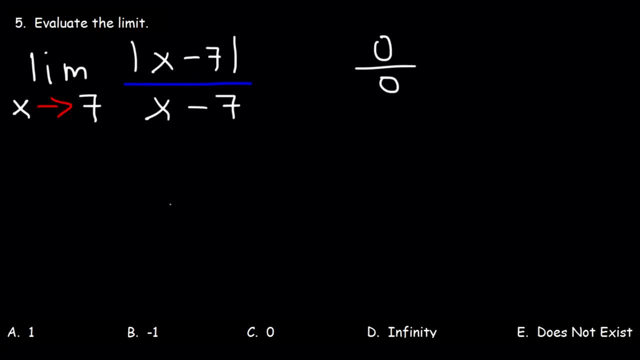 If we plug in 7, it's going to be 0 over 0, which is indeterminate, And we don't know if that's equal to 0, infinity doesn't exist- or 1 or negative 1.. So we need to check the left side and the right side of the limit. 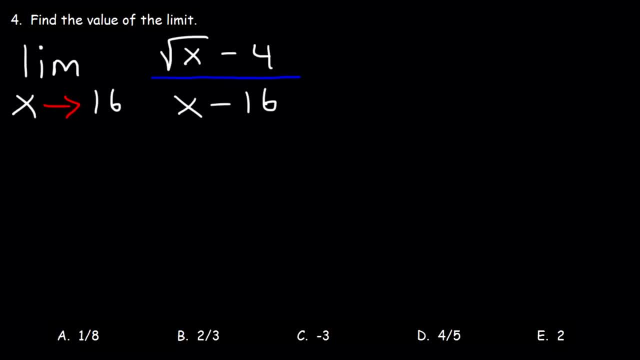 Which means c is the right answer. Number 4. Find the value of the limit. So here we have a rational function with a square root on the top. In a situation like this, we need to multiply the top and the bottom by the conjugate of the numerator. 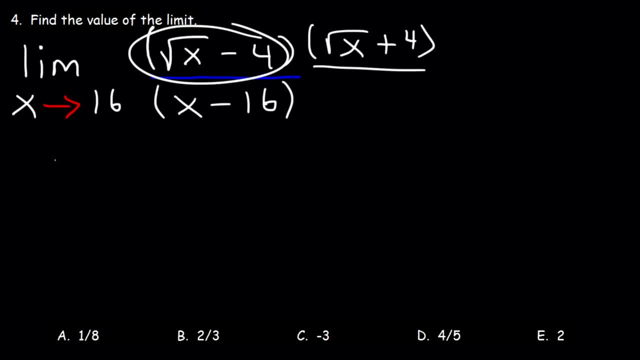 The conjugate is going to be the same thing, but you've got to change the negative sign into a positive sign, And whatever you do to the top, you must also do to the bottom. Now, on top, we're going to FOIL. 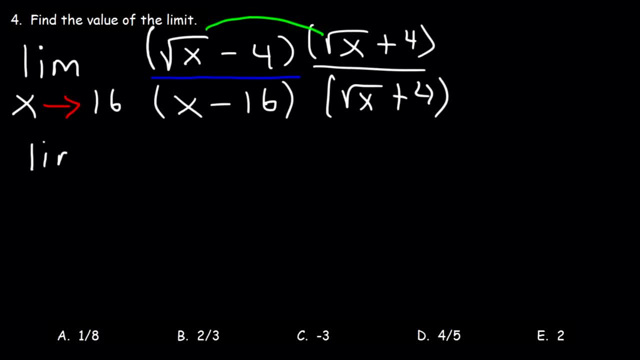 The square root of x times the square root of x is equal to x. The square root of x times 4, that's going to be positive 4 square root- x And negative 4 times the square root of x is going to be what you see here. 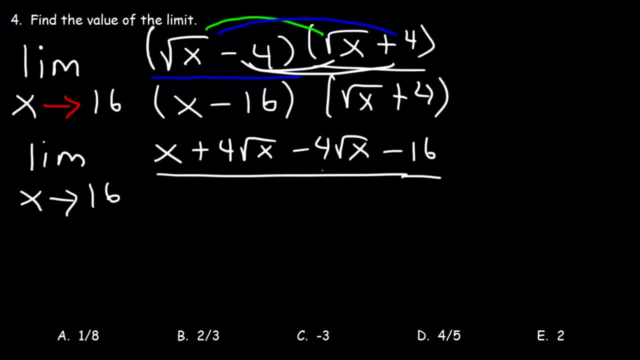 And finally we have negative 4 times 4, which is negative 16.. In a denominator, we're not going to FOIL, We're just going to rewrite what we have. So we can see that the two middle terms add up to 0, and they're going to disappear. 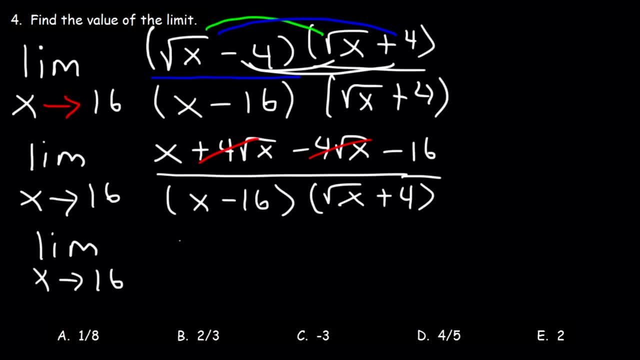 So now what we have is the limit, as x approaches 16, of x minus 16 divided by x minus 16 times the square root of x. So now we can cancel x minus 16, and at this point we can replace x with 16.. 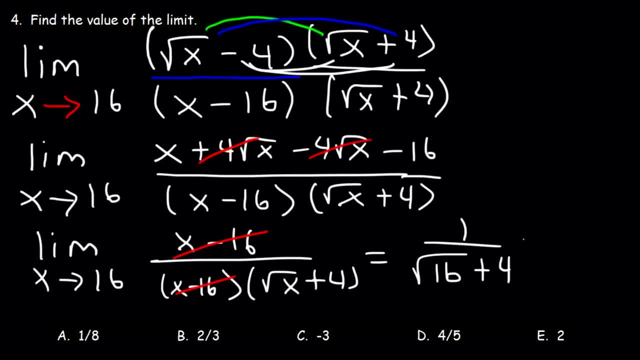 So this is going to be 1 divided by the square root of 16 plus 4.. The square root of 16 is 4, and 4 plus 4 is 8.. So the answer is 1 divided by 8, which corresponds to answer choice A. 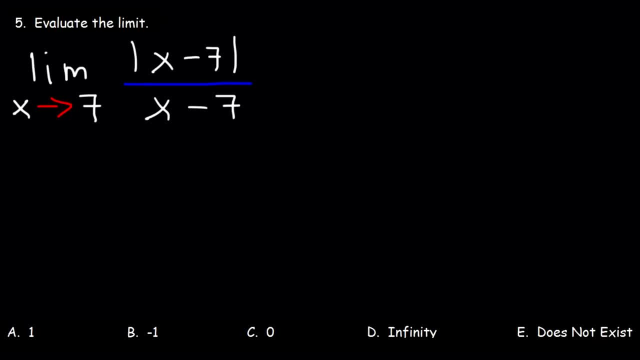 Number 5, evaluate the limit, So we can't plug in 7.. If we plug in 7, it's going to be 0 over 0, which is indeterminate, and we don't know if that's equal to 0,- infinity doesn't exist- or 1, or negative 1.. 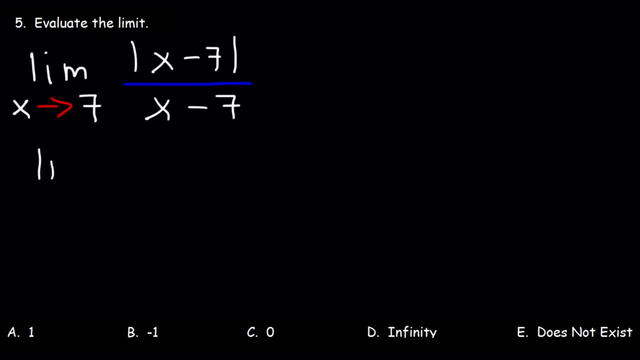 So we need to check the left side and the right side of the limit. So let's start with the left side. as x approaches 7 from the left, Let's call this f of x, So we're going to substitute a number. 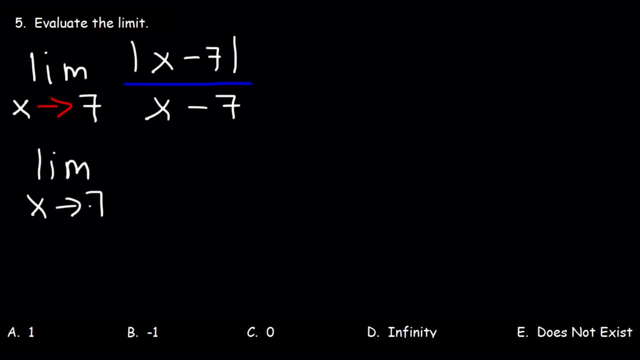 So let's start with the left side. as x approaches 7, from the left, Let's call this f of x. So we're going to substitute a number that's close to 7, but from the left, Let's use 6.9.. 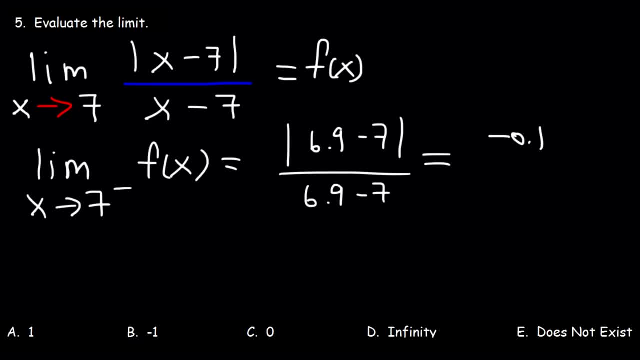 6.9 minus 7 is negative 0.1. And the absolute value of negative 0.1 is positive 0.1. And when you divide that by negative 0.1, you're going to get negative 1.. 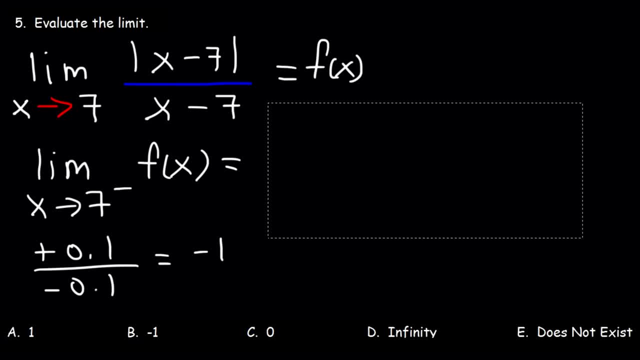 So, therefore, that is the limit. as x approaches 7 from the left, It's equal to negative 1.. Now what about from the right side? What is the limit as x approaches 7 from the right side? So let's plug in a number that's greater than 7, but close to it. 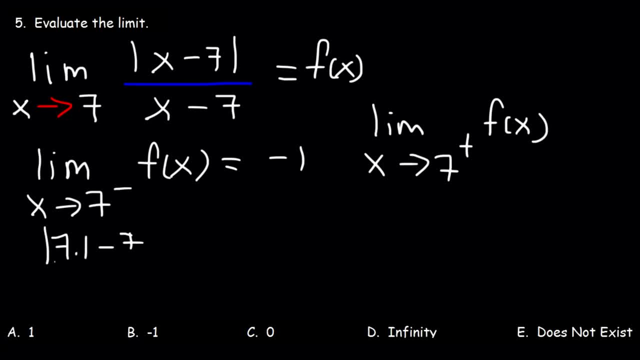 Let's try 7.1.. So 7.1 minus 7 is equal to positive 0.1. And the absolute value of positive 0.1 is positive 0.1.. Divided by itself, that's going to equal positive 1.. 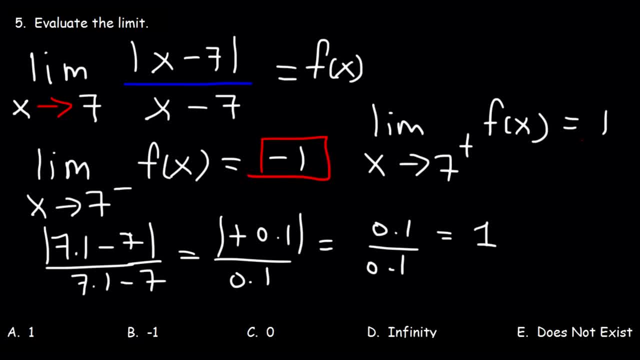 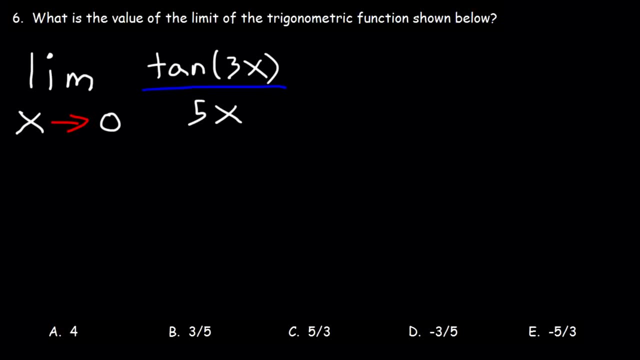 So notice that the left side and the right side do not match. So therefore the limit does not exist, Which means e is the answer Number 6.. What is the value of the limit of the trigonometric function shown below? So just by looking at it, it's going to be 3 divided by 5.. 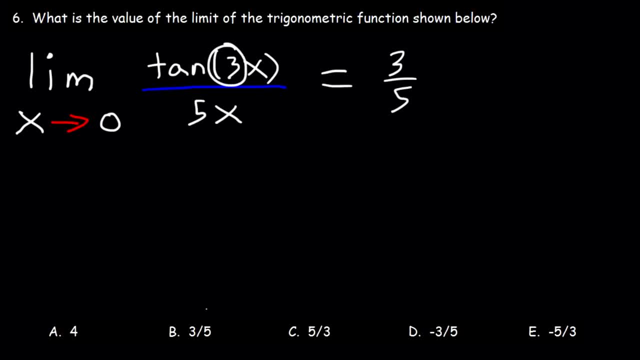 For those of you who just want a quick introduction. So it turns out, answer choice B is the right answer, But let's do some work to get our answer. So the first thing I'm going to do is I'm going to replace tangent with sine divided by cosine. 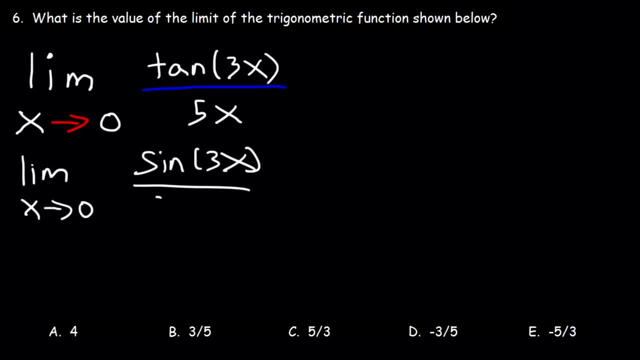 So tan 3x is sine 3x divided by cosine 3x, And we still have this 5x at the bottom, so I can write it as 1 over 5x. Now what I need to have under sine 3x is a 3x. 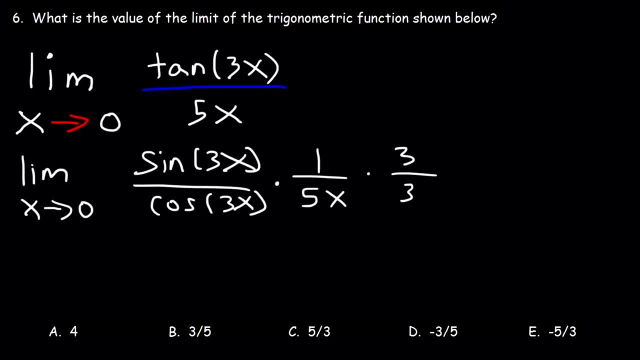 I'm going to multiply the top and the bottom by 3.. So I'm going to trade places with the cosine and the 3. I'm also going to move the x in that position as well. So this is all equal to the limit as x approaches 0.. 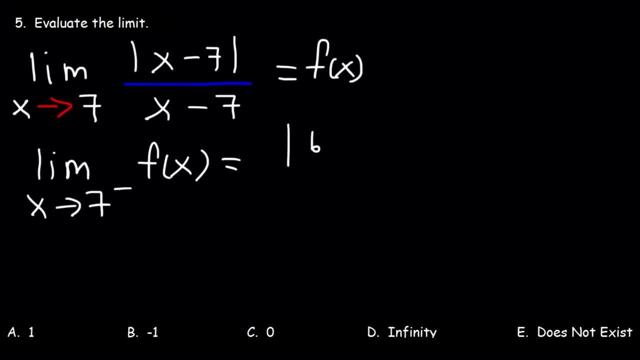 That's going to be x. That's close to 7, but from the left Let's use 6.9.. 6.9 minus 7 is negative 0.1.. And the absolute value of negative 0.1 is positive 0.1.. 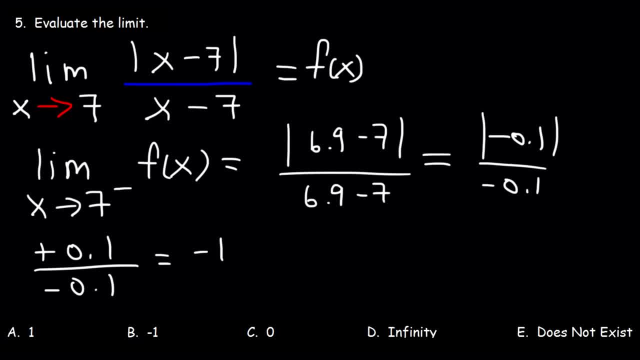 And when you divide that by negative 0.1, you're going to get negative 1.. So therefore, that is the limit. as x approaches 7 from the left side, It's equal to negative 1.. Now what about x? 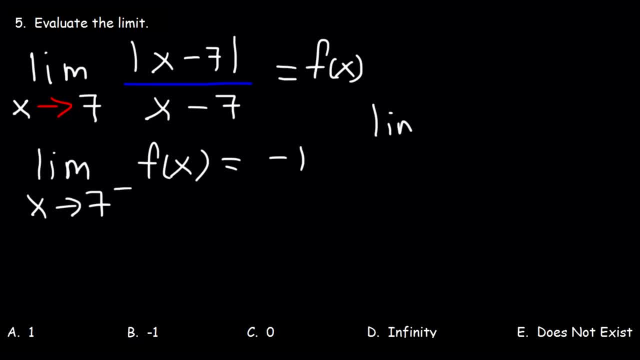 What about from the right side? What is the limit as x approaches 7 from the right side? So let's plug in a number that's greater than 7, but close to it. Let's try 7.1.. So 7.1 minus 7 is equal to positive 0.1. 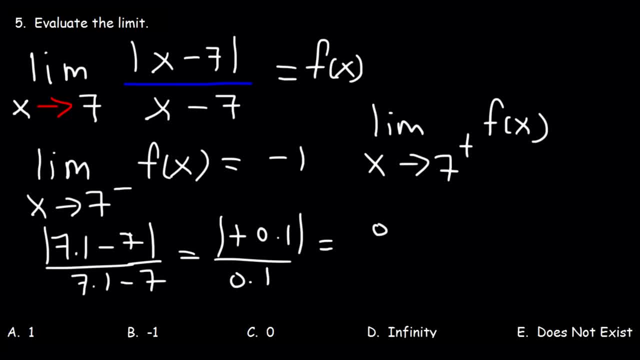 And the absolute value of positive 0.1 is positive 0.1.. Divided by itself, That's going to equal positive 1. So notice that the left side and the right side do not match, So therefore the limit does not exist. 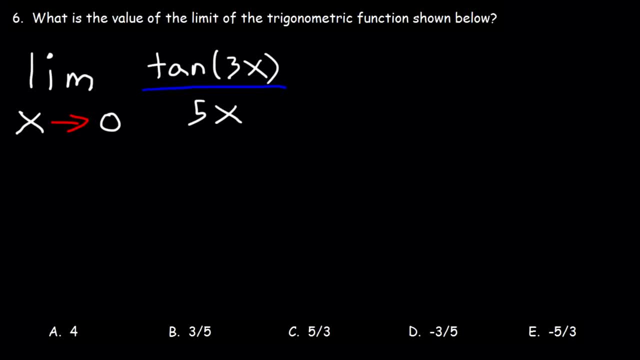 Which means E is the answer Number 6.. What is the value of the limit of the trigonometric function shown below? So, just by looking at it, it's going to be 3 divided by 5.. For those of you who just want a quick answer, 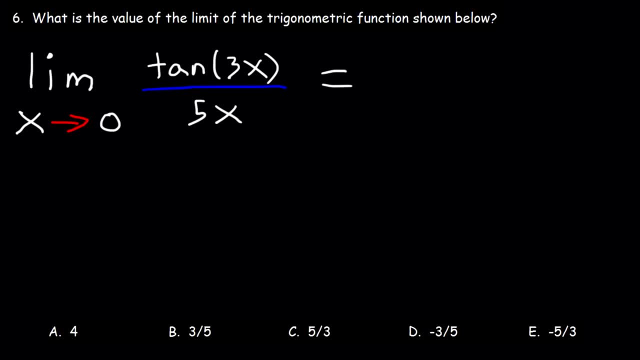 So it turns out, Answer choice B is the right answer, But let's do some work to get our answer. So the first thing I'm going to do is I'm going to replace tangent with sine divided by cosine. So tan 3x is sine 3x divided by cosine 3x. 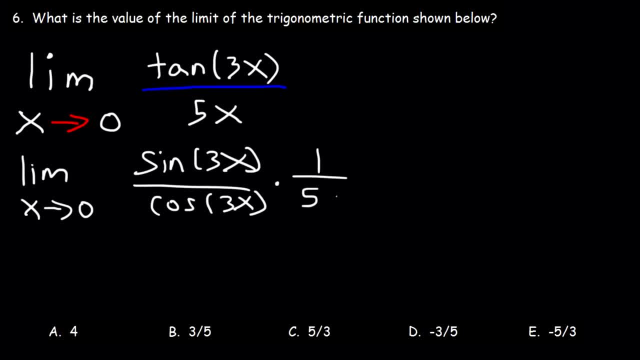 And we still have this 5x at the bottom, So I can write it as 1 over 5x. Now what I need to have under sine 3x is a 3x. I'm going to multiply the top and the bottom by 3x. 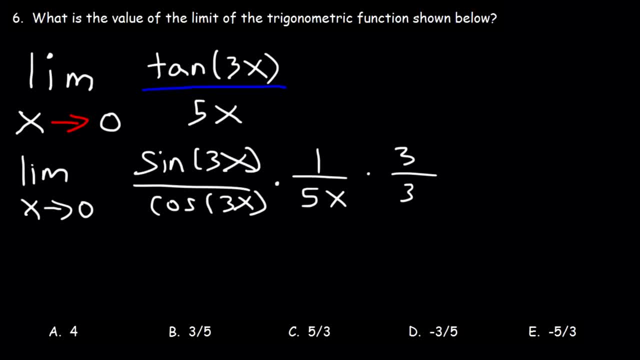 Sweep that down to 3.. So I'm going to trade places with the cosine and the 3.. I'm also going to move the x in that position as well. So this is all equal to the limit as x approaches 0.. Sine 3x divided by 3x times the limit as x approaches 0. 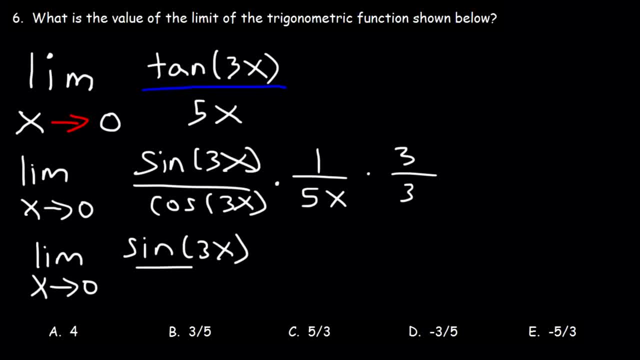 Sine 3x divided by 3x times the limit as x approaches 0.. I still have a 3 on top And I've already moved the 3x to the left. So on the bottom I have a 5 and a cosine 3x. 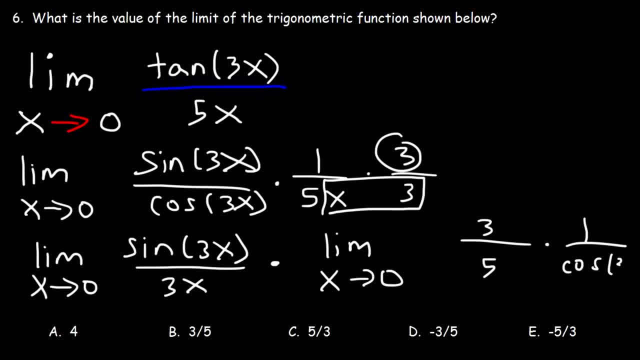 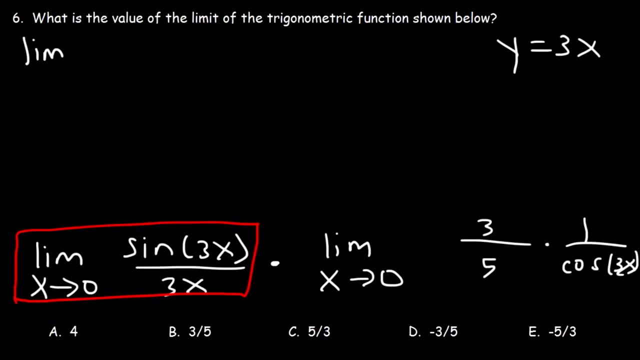 Which I'm going to write as 1 over cosine 3x. So now I'm going to use substitution. Let's say that y is equal to 3x. So therefore this limit expression becomes the following expression: The limit as y approaches 0 of sine y divided by y. 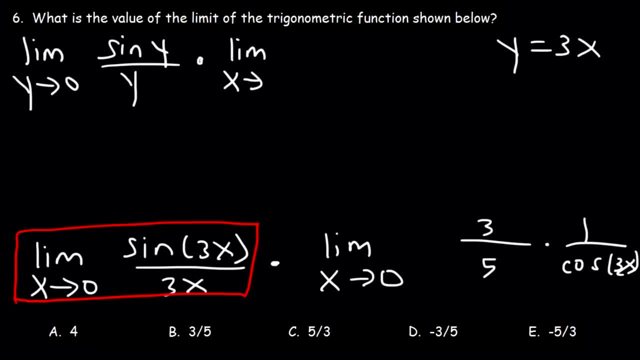 Times the limit as x approaches 0. And here this is a function based on x. So this is going to be 1 over cosine, 3x times 3 over 5.. Now the limit as y approaches 0.. The limit as y approaches 0 of sine y divided by y. 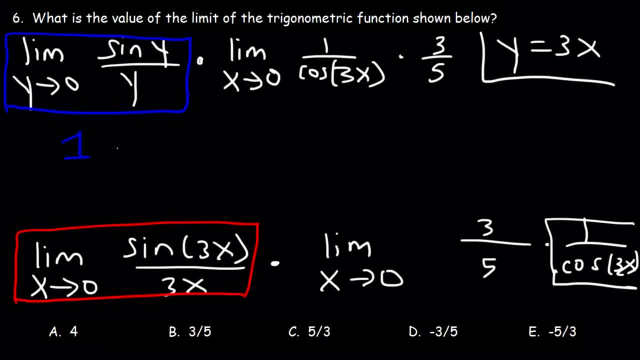 That's equal to 1.. You just need to know that formula. You can always plug in a small value of x And you can confirm that as 1.. Cosine 0: if we replace x with 0.. 3 times 0 is still 0.. 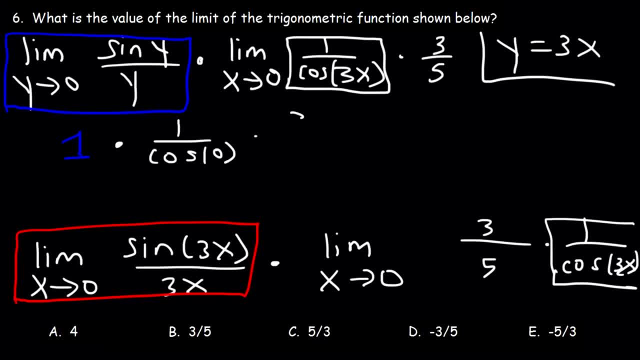 Cosine 0 is equal to 1.. But I'll replace that in the next step. So what we have is 1 times 1 times 3 over 5., Which gives us a 4.. So we have a final answer of 3 divided by 5.. 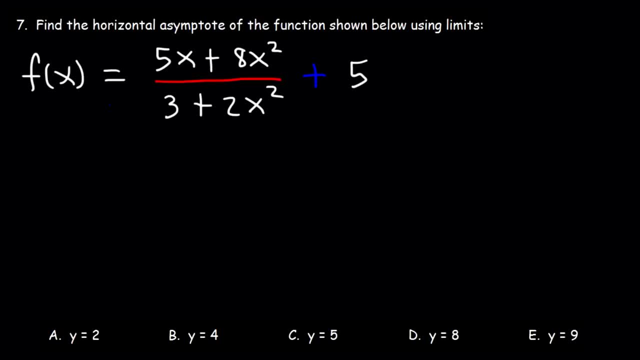 So, therefore, answer choice B is the right answer, Number 7.. Find the horizontal asymptote of the function shown below using limits. To do so we need to find the limit as x approaches infinity Of the function, 5x plus 8x squared. 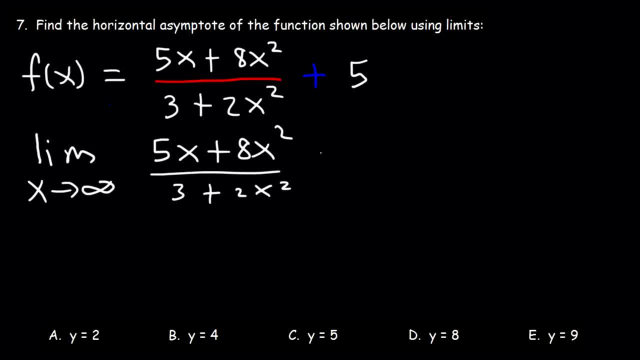 Divided by 3x plus 2x squared plus 5.. Now keep in mind when x becomes very large, 5x is insignificant compared to 8x squared If you replace x with 1000.. 5000 is not significant to 8 million. 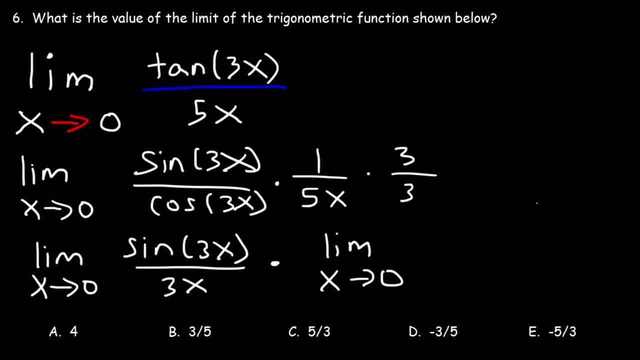 Simple: 3x, 2x, 3x. I still have 2x, 3x, 3x, 4x, 4x, 4x, 4x, have a 3 on top and I've already moved the 3x to the left. so on the bottom I have a 5 and a cosine 3x. 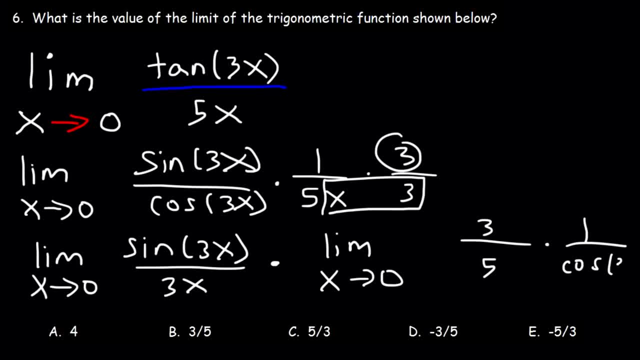 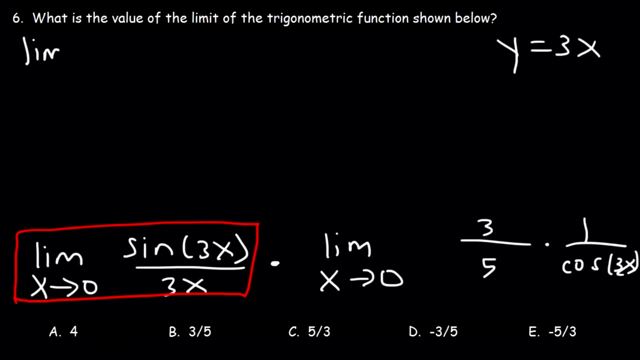 which I'm going to write as 1 over cosine 3x. So now I'm going to use substitution. Let's say that y is equal to 3x, So therefore this limit expression becomes the following expression: The limit as y approaches 0 of sine y divided by y times the limit as x approaches 0,, and here this is a. 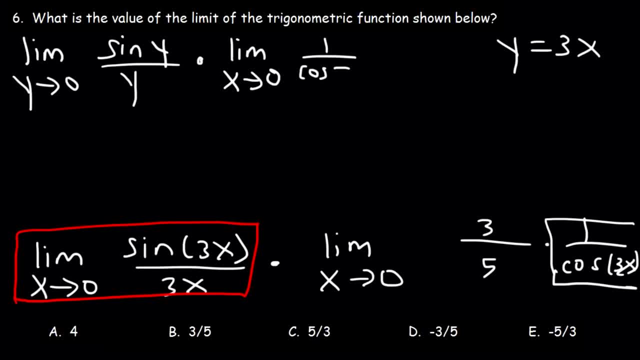 function based on x. so this is going to be 1 over cosine 3x times 3 over 5.. Now the limit as y approaches 0 of sine y divided by y, that's equal to 1.. You just need to know that formula. 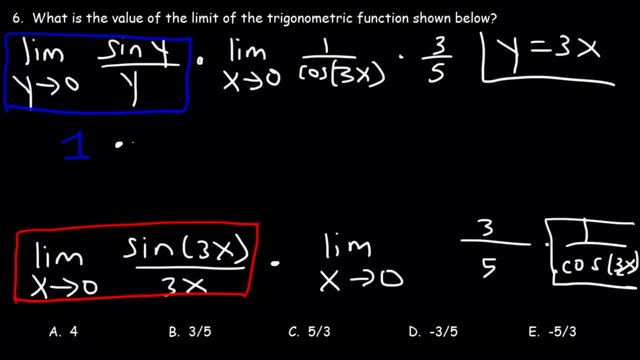 You can always plug in a small value of x and you can confirm that it's 1.. Cosine 0,: if we replace x with 0,, 3 times 0 is still 0. Cosine 0 is equal to 1, but I'll replace that in the next step. So what we have is 1 times 1 times 3 over 5.. 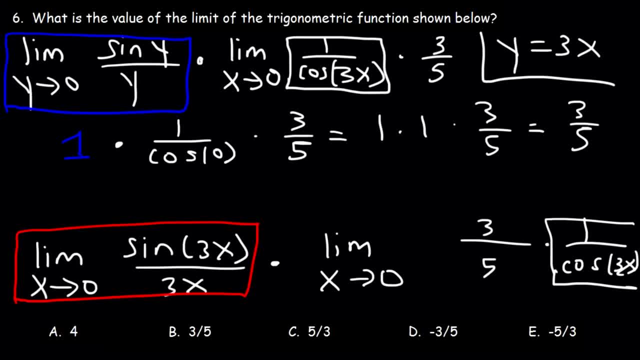 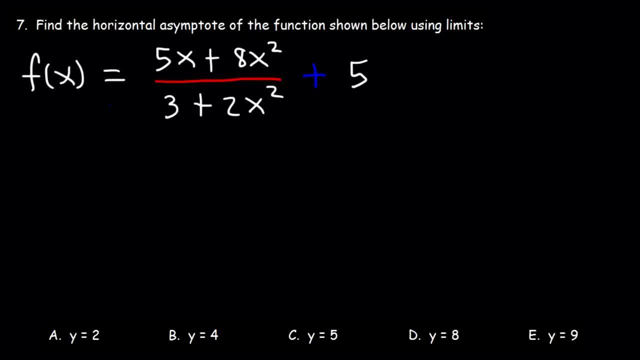 Which gives us a final answer of 3 divided by 5.. So, therefore, answer choice B is the right answer. Number 7.. Find the horizontal asymptote of the function shown below using limits. To do so we need to find the limit, as x approaches infinity, of the function, 5x plus 8x squared. 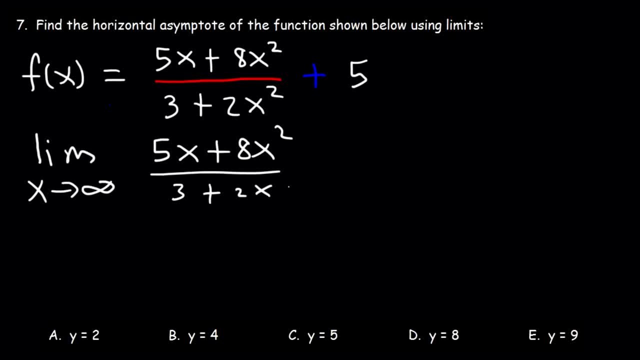 divided by 3x plus 2x squared plus 5.. Now keep in mind when x becomes very large, 5x is insignificant compared to 8x squared. If you replace x with 1000,, 5000 is not significant to 8 million and 3 is not significant to 2 million. 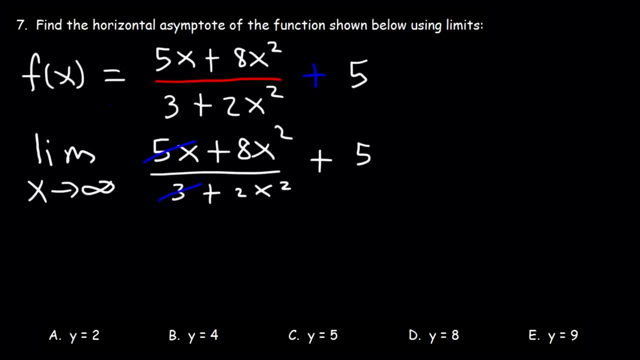 And 3 is not significant to 2 million, So therefore this expression becomes equivalent to the limit, as x approaches infinity, Of 8x squared divided by 2x squared plus 5.. You can only do this when x approaches infinity And x becomes very large. 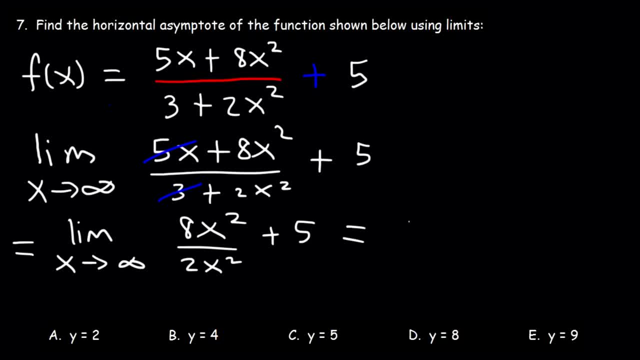 Mathematically it works out: 8 divided by 2 is 4.. And you can cancel the x squared because they are the same. So what we now have is 4 plus 5. Which is equal to 9.. So therefore, 9 is the final answer. 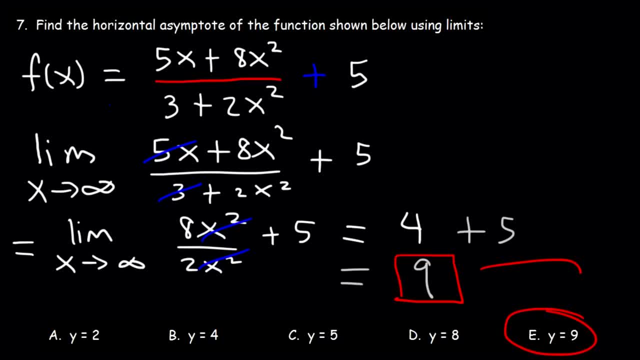 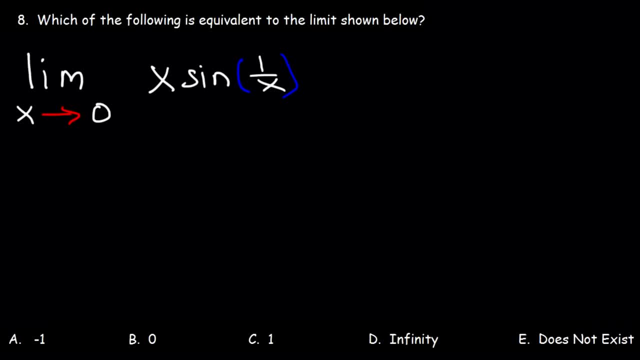 And that's going to be the horizontal asymptote. It's an equation: Y equals 9.. So E is the right answer, Number 8.. Which of the following is equivalent to the limit shown below? So go ahead and take a minute and try this problem. 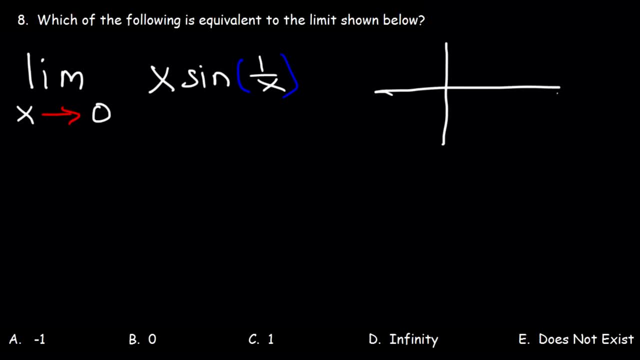 Now what you need to know is that the sine function oscillates between 1 and negative 1.. This is the graph of sine x. Now, the only difference between sine x and sine 1 over x Is how fast it oscillates As you approach an x value of 0.. 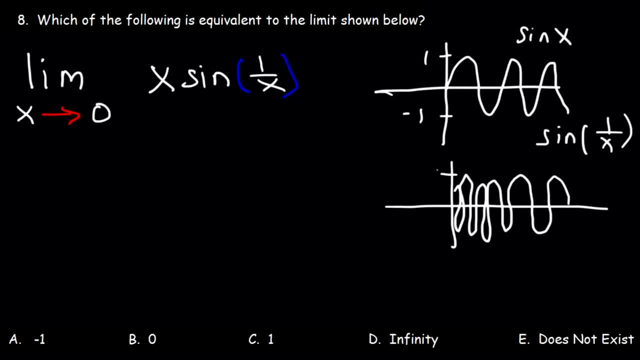 It begins to oscillate faster and faster. However, The amplitude still varies between 1 and negative 1.. So it really doesn't matter The angle Or the fact that we have a 1 over x Within sine, Because as x approaches 0.. 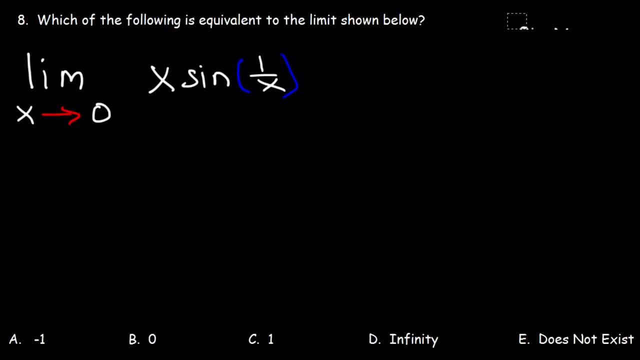 1 over x does not exist. As x approaches 0 from the left, 1 over x becomes Negative infinity. And as x approaches 0 from the right, 1 over x becomes positive infinity. But that doesn't matter for the sine function. 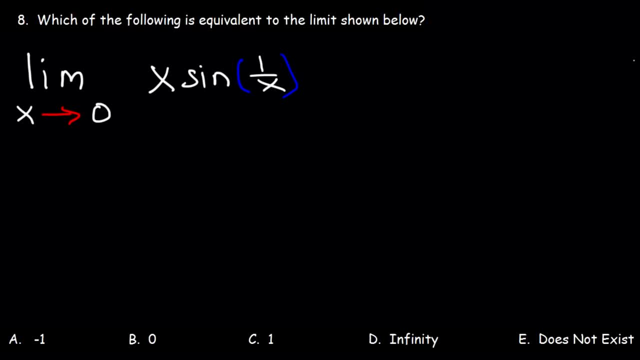 Because it's always going to alternate Between 1 and negative infinity, Because it's always going to alternate Between negative 1 and 1.. So we can make this statement: Sine of 1 over x Will always be between. 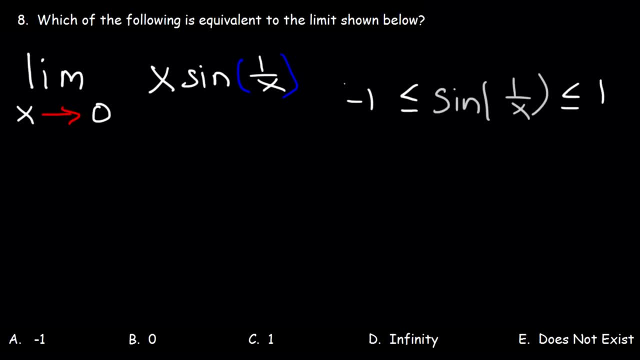 Negative 1 and 1.. Now if we multiply Everything by x, We can get this expression: Negative x Is between sine, Is between x, Sine, 1 over x And 1 over x, And it's between 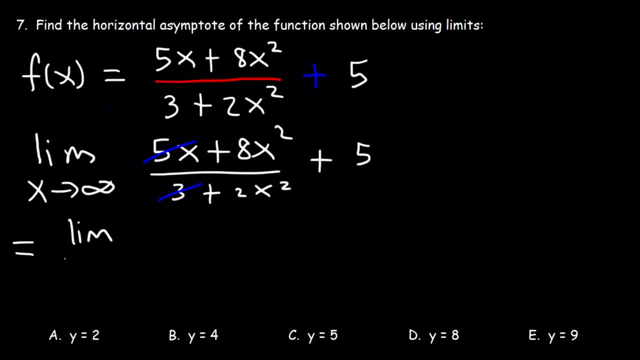 So therefore, this expression becomes equivalent to the limit, as x approaches infinity, of 8x squared divided by 2x squared plus 5.. You can find this expression in the next step. only do this when X becomes very large. Mathematically, it works out 8 divided by 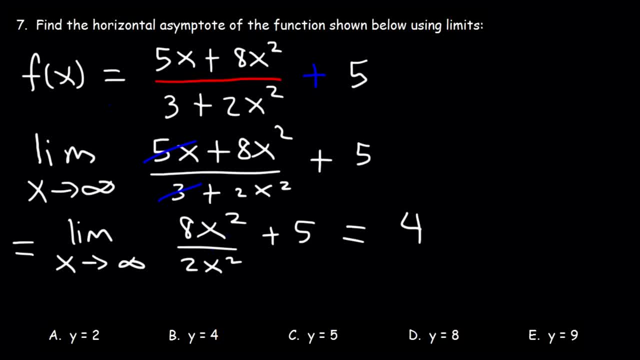 2 is 4, and you can cancel the x-squares because they're the same. So what we now have is 4 plus 5, which is equal to 9.. So, therefore, 9 is the final answer, and that's going to be the horizontal asymptote. It's an equation: y equals 9,, so 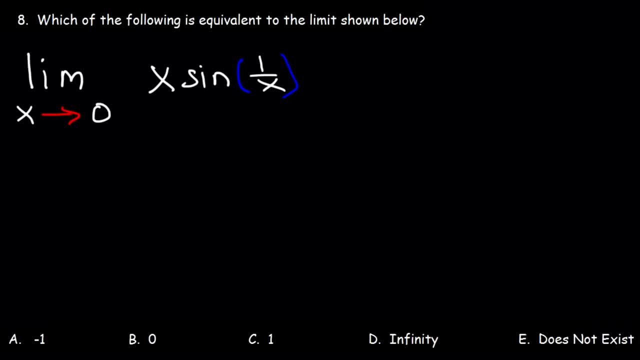 E is the right answer, Number 8.. Which of the following is equivalent to the limit shown below? So go ahead, take a minute and try this problem Now. what you need to know is that the sine function oscillates between 1 and negative 1. This 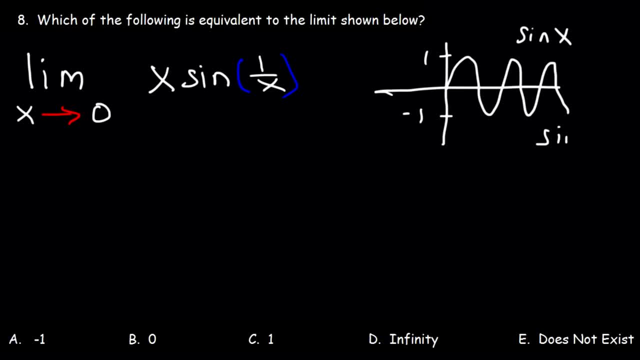 is the graph of sine X. Now. the only difference between sine X and sine 1 over X is how fast it oscillates. As you approach an X value of 0, it begins to oscillate faster and faster. However, the amplitude still varies. 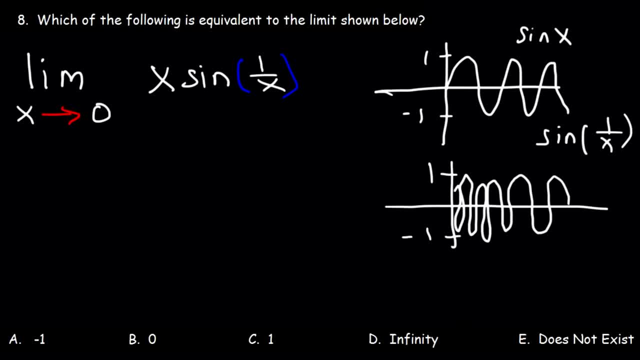 between 1 and negative 1.. So it really doesn't matter the angle or the fact that we have a 1 over X within sine, because as X approaches 0, 1 over X does not exist. As X approaches 0 from the left, 1 over X becomes negative. 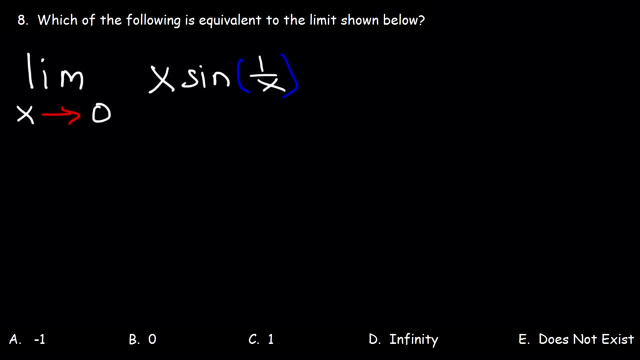 infinity. and as X approaches 0 from the right, 1 over X becomes negative. infinity over x becomes positive infinity. But that doesn't matter for the sine function, because it's always going to alternate between negative 1 and 1.. So we can make this statement Sine. 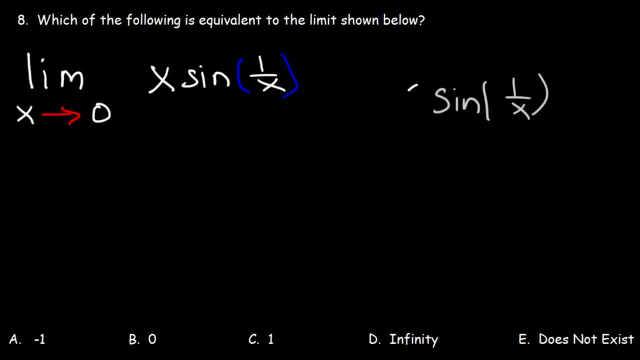 of 1 over x will always be between negative 1 and 1.. Now if we multiply everything by x, we can get this expression: Negative x is between x sine 1 over x and it's between positive x. So x sine 1 over x is between negative x and positive x. That's what I meant. 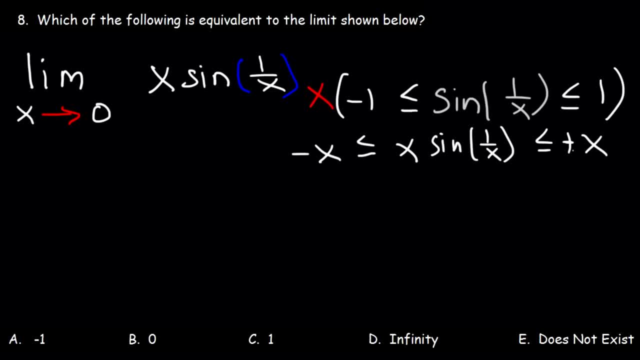 Positive x. So x Sine 1 over x Is between negative x and positive x. Now what we can use Is the squeeze term. So basically, The squeeze term states that Let's call this h of x And let's say f of x. 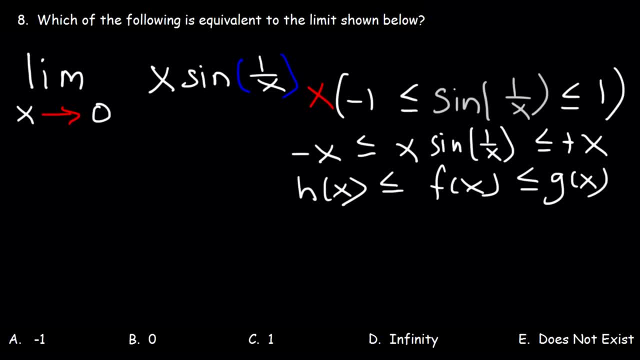 Is between h of x and g of x, If the limit As x approaches 0.. H of x and g of x. If they're the same, Then the limit as x approaches f of x Must also be the same. So that's the main idea behind the squeeze term. 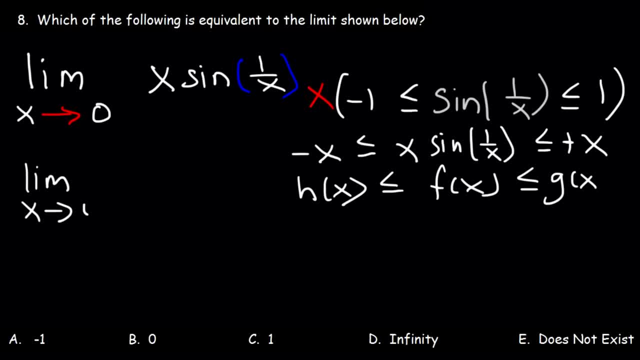 So the limit As x approaches 0.. For h of x, Which is really negative x, Well, that's equal to 0.. Now the limit As x approaches 0.. Of g of x, Which in this case is positive x. 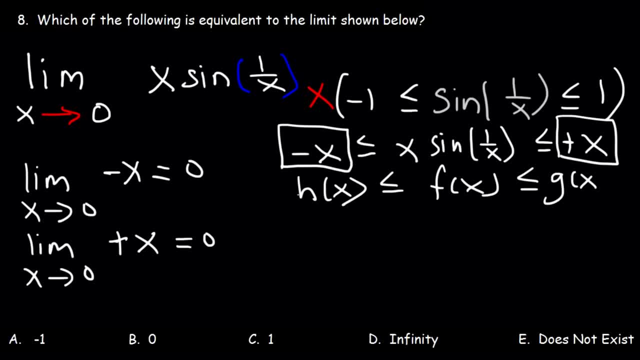 That too Is equal to 0. So therefore, the limit As x approaches x sine of 1 over x. Since it's between Negative x and x, It too Must also equal 0. So therefore, b Is the right answer. 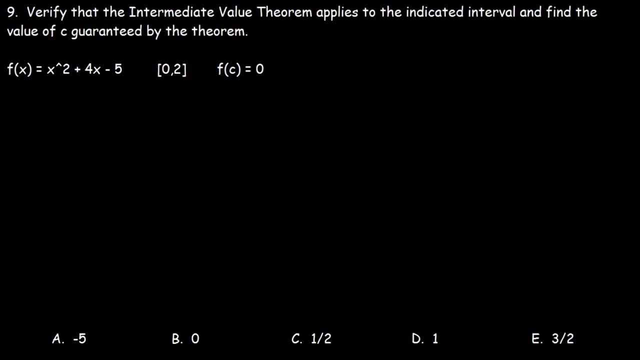 According to the squeeze term, Number 9.. Verify that the intermediate value theorem Applies to the indicated interval And find the value of c Guaranteed by the theorem. So Based on the intermediate value theorem. You need to know that It states that: 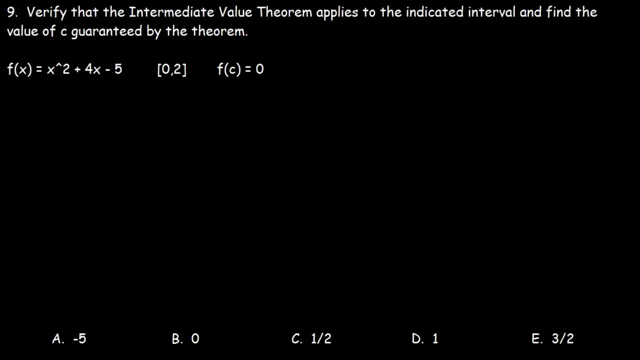 f has to be continuous On the closed interval a to b And that f of a Cannot equal f of b, And there is Some number, k, Which is between f of a And f of b, Such that 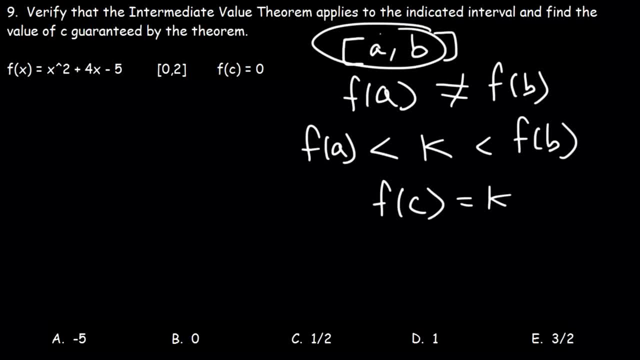 f of c Is equal to k And c Has to be in the interval Of a and b. So We got to find That value of c, Such that k Is between f of a and f of b. Notice that we have the value of k. 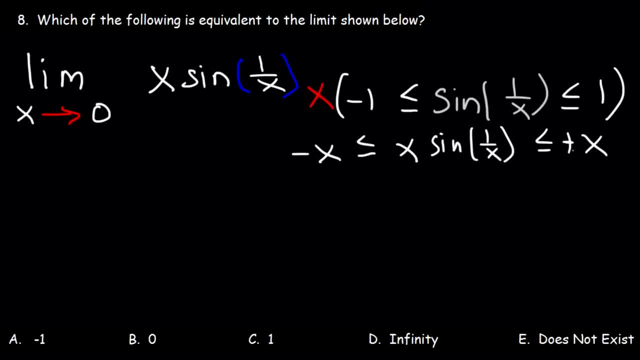 to say. Now, what we can use is the squeeze term. So basically, the squeeze term states that let's call this h of x and let's say f of x is between h of x and g of x. If the limit as x approaches 0 of h of x and g of x- if they're the same- then the limit as x approaches. 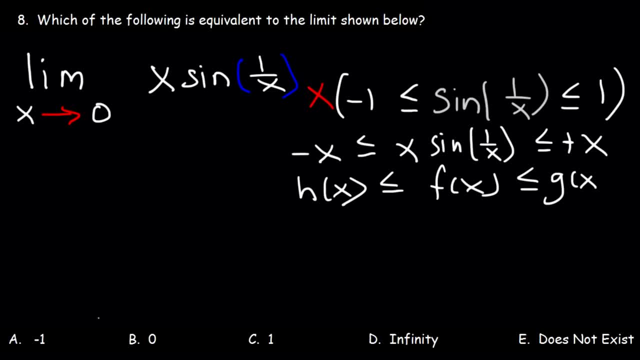 f of x must also be the same. So that's the main idea behind the squeeze term. So the limit as x approaches 0 for h of x, which is really negative x, well, that's equal to 0.. Now the limit as x approaches 0 of g of x, which in this case is positive x, that too. 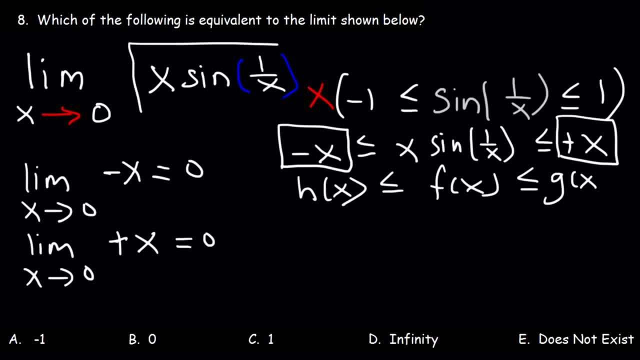 is equal to 0.. So therefore, the limit as x approaches x sine of 1 over x. since it's between negative x and x, it too must also equal 0. So therefore, b is the right answer according to the squeeze term. 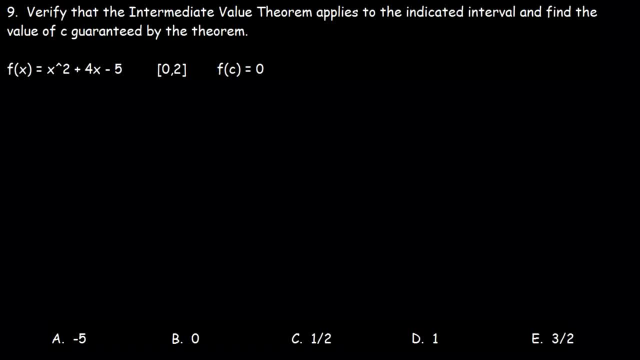 Number nine: verify that the intermediate value theorem applies to the indicated interval and find the value of Z guaranteed by the theorem. So, based on the intermediate value theorem, you need to know that it states that f has to be continuous on the closed interval a to b and that f cannot equal f. 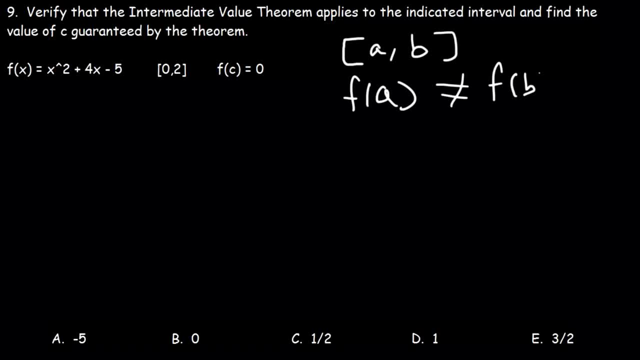 B and there is some number, K, which is between F of A and F of B, such that F of C is equal to K and C has to be in the interval of A and B. so we got to find that value of C, such that K is between F of A and F of B. notice that we 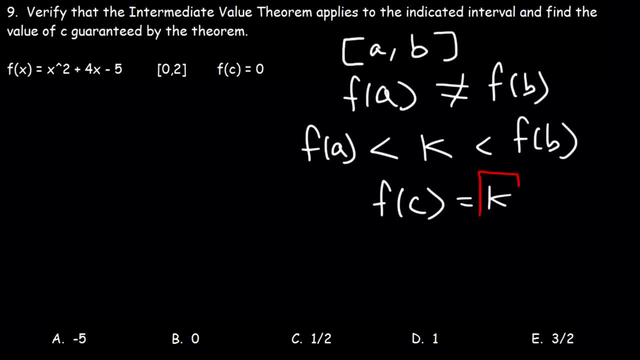 have the value of K. K is whatever number F of C is equal to. so therefore K is 0. so first we got to show that F of A and F of B. well, we have to show that 0 is between F of A and F of B. we have to prove that the IVT theorem applies. so 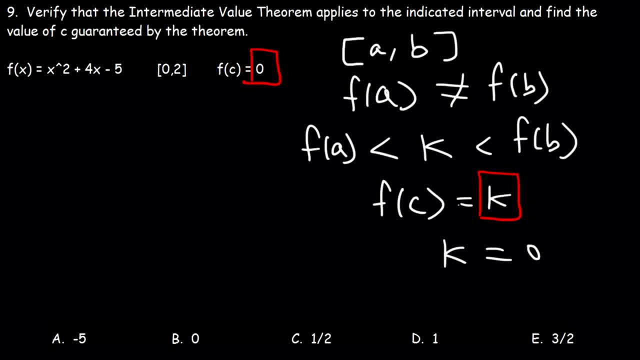 Is zero. So first We got to show that f of a and f of b. Well, we have to show that zero Is between f of a and f of b. We have to prove that the IVT theorem applies. So let's find f of a. 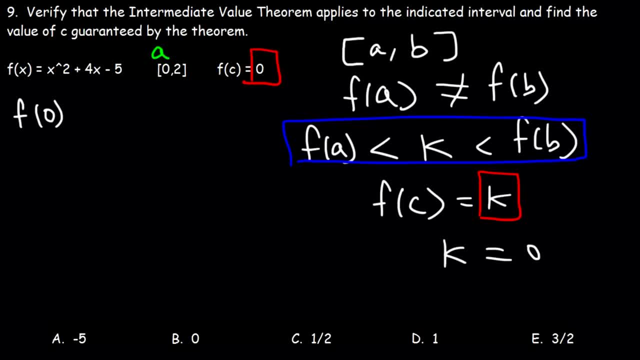 Where a is zero And b is two. So f of zero Is going to be zero squared Plus four times zero Minus five, And zero is negative five. Now Let's calculate f of b, Which is f of two. 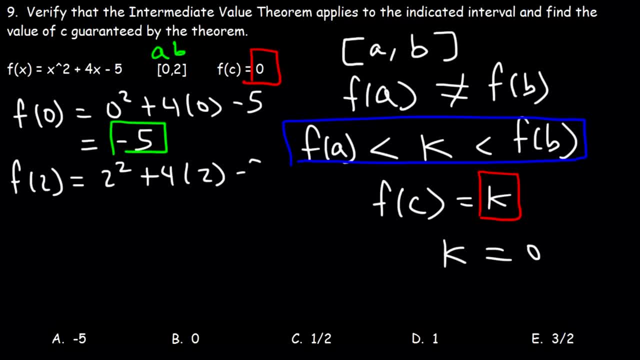 So that's going to be two squared Plus four times two Minus five. Two squared is four. Four times two is eight. Four plus eight is twelve Minus five, That's seven. So the intermediate value theorem Does apply to the indicated interval. 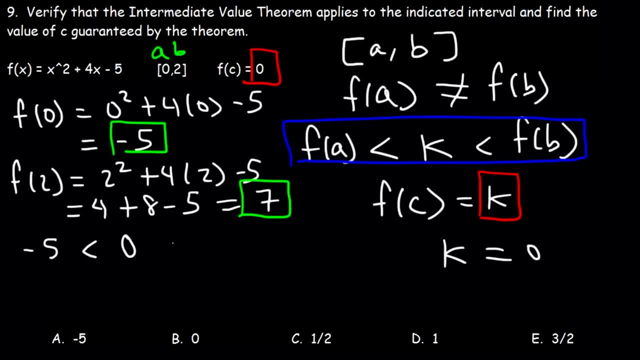 As we can see, Is in between negative five And seven. So now that we know that the IVT Theorem applies, We can now find the value of c. So let's set f of c Equal to zero, So basically set the function f of x. 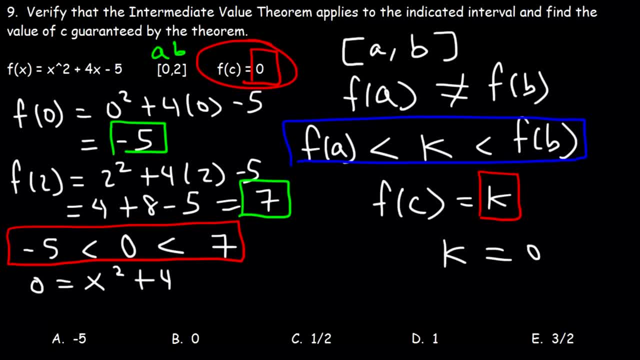 Replace it with zero And find the value of x. So zero is equal to x squared Plus four, x minus five. Now we need to factor Two numbers that multiply to negative five. That's a positive four Are positive five and negative one. 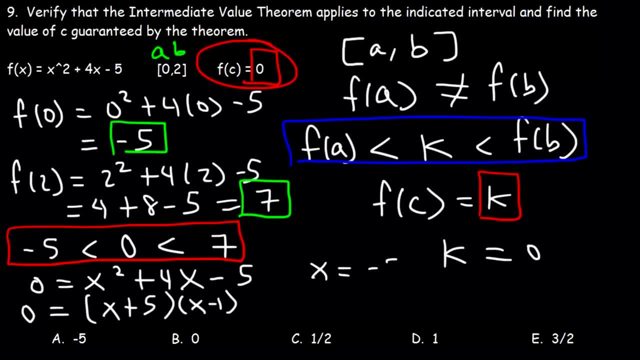 Therefore, We can see that x is equal to negative five And positive one. If you reverse the signs, If you set x plus five equal to zero, X will equal negative five, And if you set x minus one equal to zero, X will equal positive one. 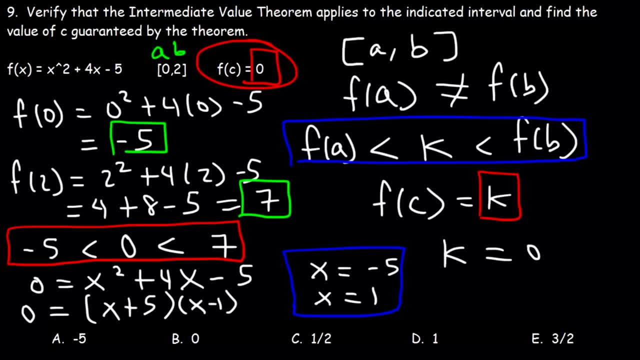 Now, one of these values Is the c value That we're looking for, So c has to be in the interval A to b, Between zero and two. Negative five is not between zero and two, But one is, So therefore c. 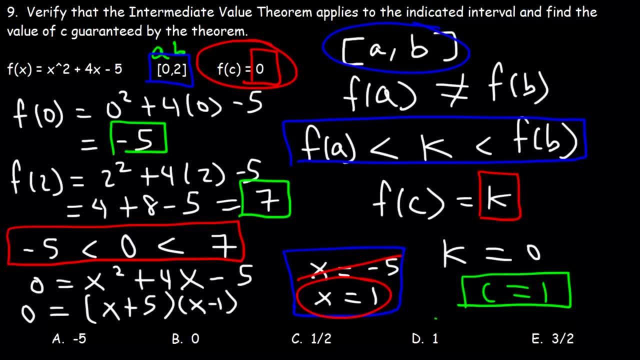 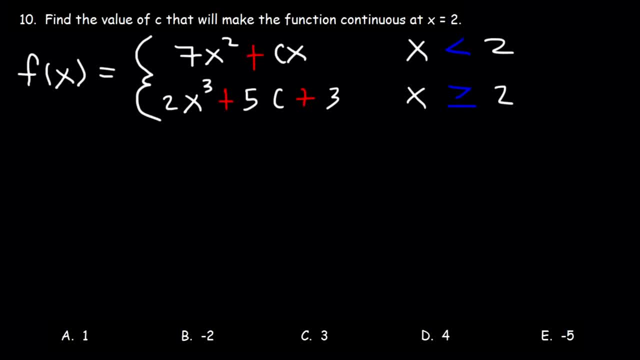 Is equal to one, Which means d Is the right answer. Number ten: Find the value of c That will make the function continuous At x equals two. The first thing we need to do Is set these two functions equal to each other. 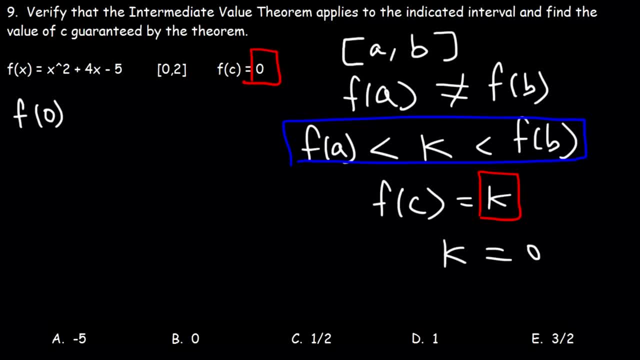 let's find F of A, where A is 0 and B is 2. so F of 0 is going to be 0 squared plus 4 times 0 minus 5. so F of 0 is negative 5. now let's calculate F of B, which is F of 2. so 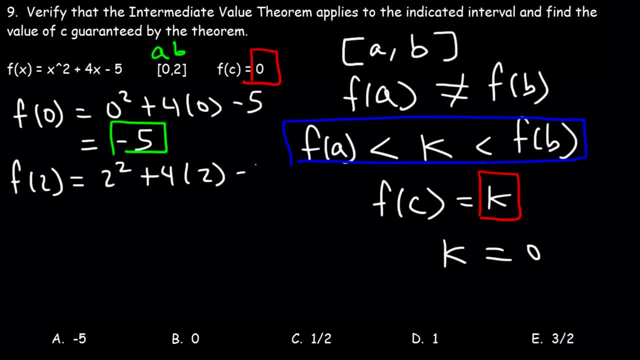 that's going to be 2 squared plus 4 times 2 minus 5. 2 squared is 4, 4 times 2 is 8. 4 plus 8 is 9, so that's 8 is 12 minus 5, that's 7. so the intermediate value theorem does. 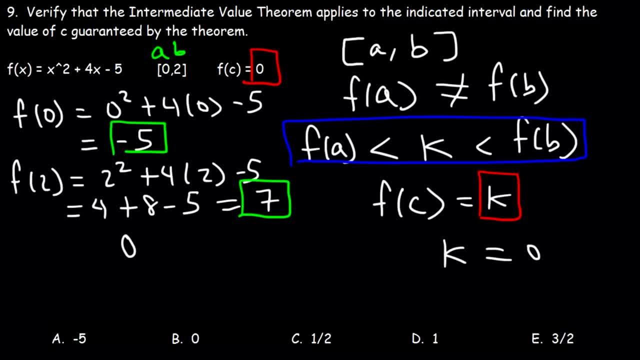 apply to the indicated interval. as we can see, K, which is 0, is in between negative 5 and 7. so now that we know that the IVT theorem applies, we can now find the value of C. so let's set F of C equal to 0, so basically set the. 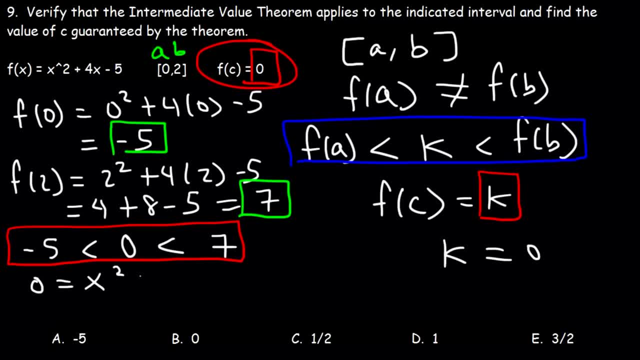 Set the function f of x, replace it with 0, and find the value of x. So 0 is equal to x squared plus 4x minus 5.. Now we need to factor Two numbers that multiply to negative 5 but add to positive. 4 are positive, 5 and negative. 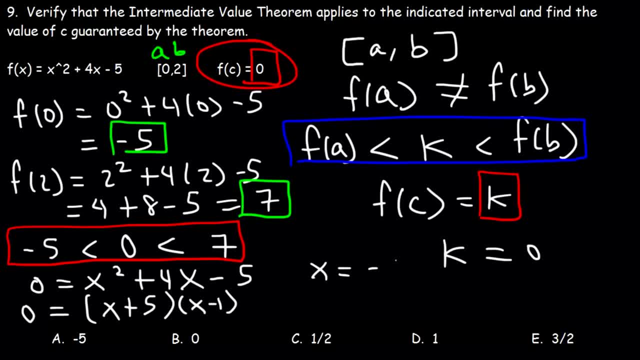 1.. Therefore, we can see that x is equal to negative 5 and positive 1. if you reverse the signs, If you set x plus 5 equal to 0, x will equal negative 5.. And if you set x minus 1 equal to 0,, x will equal positive 1.. 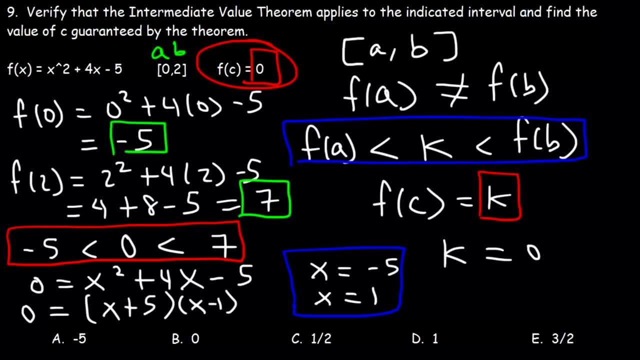 Now, one of these values is the c value that we're looking for, So c has to be in the interval a to b, that is, between 0 and 2.. Negative 5 is not between 0 and 2, but 1 is. 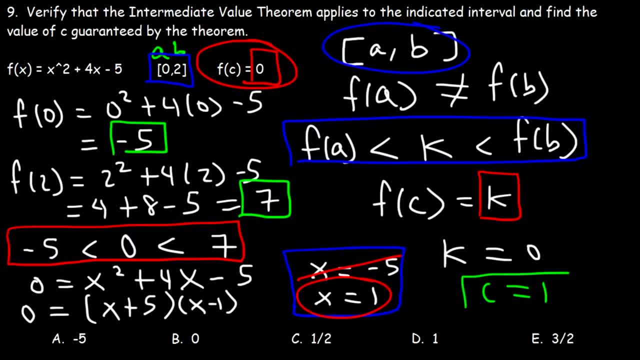 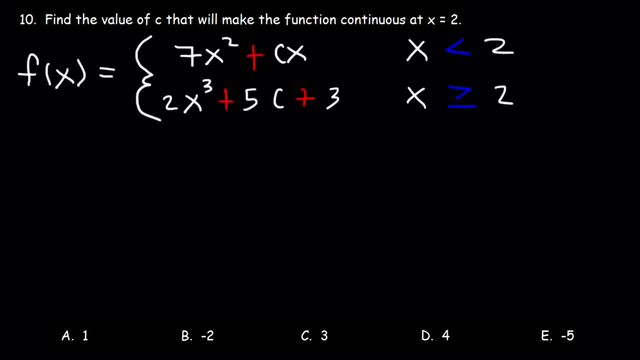 So therefore, c is equal to 1, which means d is the right answer Number 10.. Find the value of c that will make the function continuous at x equals 2.. The first thing we need to do is set these two functions equal to each other.